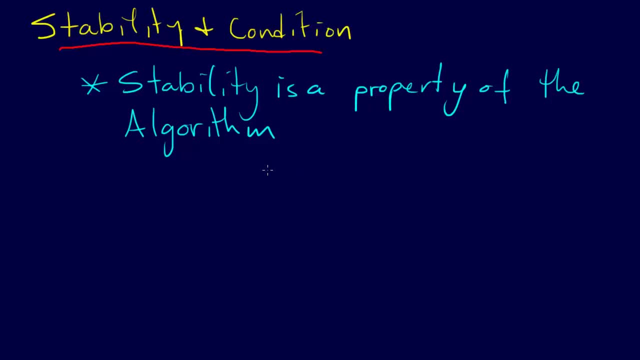 grossly magnify. errors that were present in the input aren't grossly magnified into the output. That is stability, numerical stability, and that is a property of the algorithm. If an algorithm doesn't perform well on this, it's called numerically unstable. 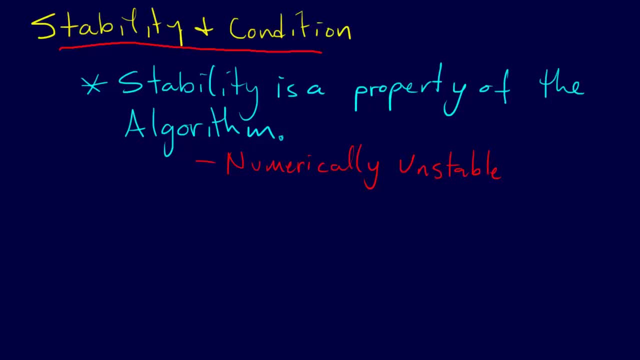 Again, this is a property of the algorithm. On the other hand, we have condition, We have condition, and condition is a property of the algorithm. Not of the algorithm, but of the problem itself. And so this is where we have errors in the input, and the input may lead to gross errors in the output. 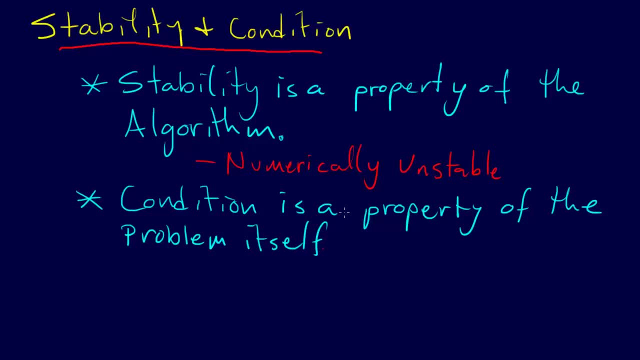 but not necessarily as a result of the algorithm. We may have errors in the input, but not necessarily as a result of the algorithm. very stable algorithm and yet we may still, even with slight errors in the input, have gross errors in the output. 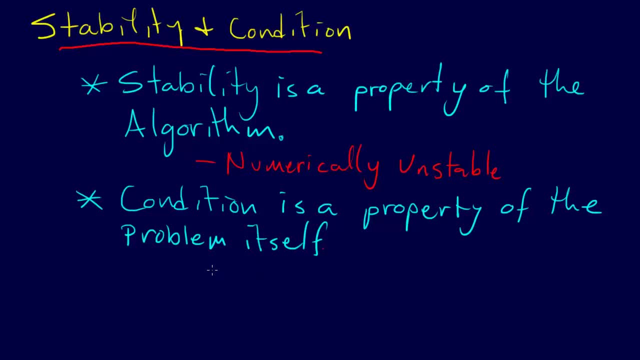 And that is a property called the condition and it's a property of the problem itself. and if the problem is poor we call that problem ill-conditioned. And obviously worst case is if we have both an ill-conditioned problem and we're using 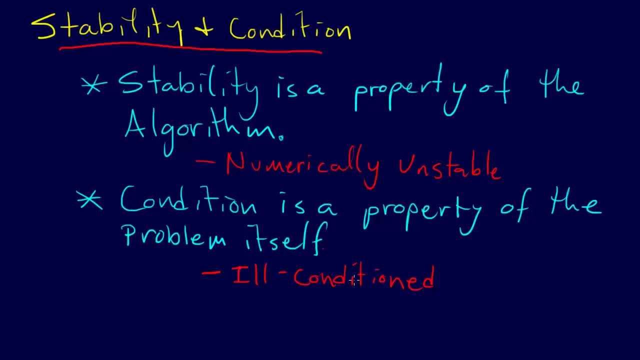 a numerically unstable algorithm. those are both things that we want to avoid. Unfortunately, there's not always anything we can do about the condition of the problem. Sometimes there is, and so we can sometimes do some things, But this is important to note. 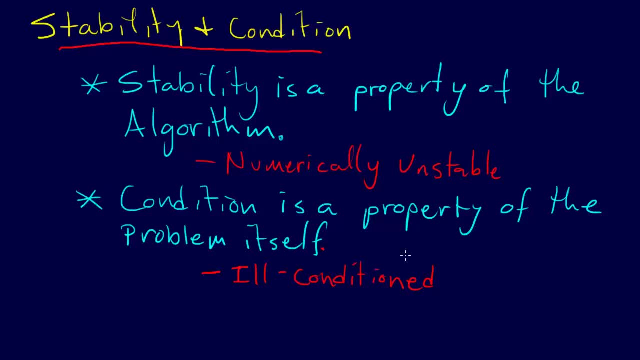 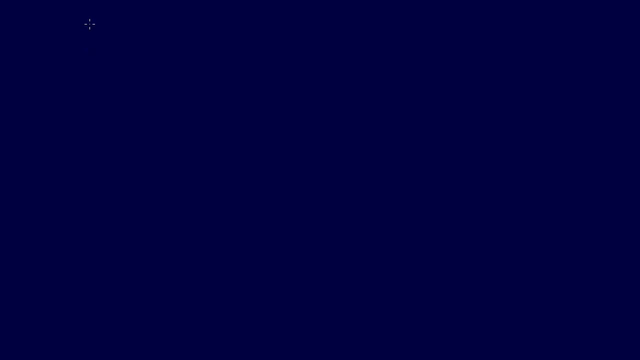 And there is a way that we can define something called the condition number, And they do this in the book: Condition number. So let's delve into this a little bit, but not too much, Because I don't want us to get. 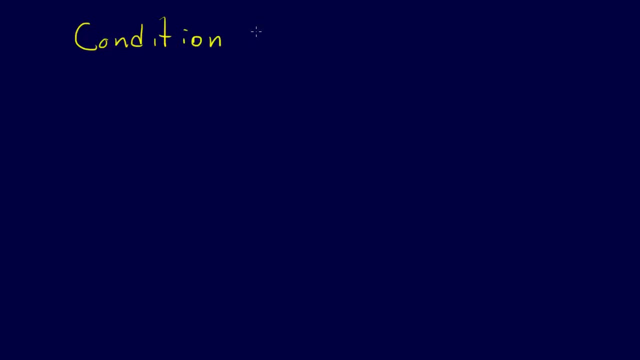 I want you to know how to do a little bit of analysis on this, but I don't want you to get too hung up on this. the condition number And they derive this in the book And they basically they look at the relative of the error in y. so error in y they take. 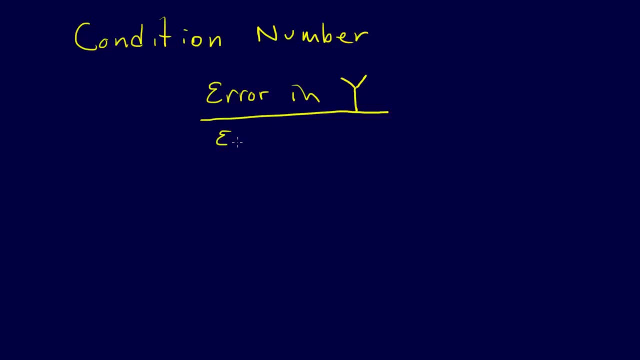 the ratio of the error in y to the error in x, error in x- And this is relative error that we talked about before. So that'd be like y minus y over y true right And x minus louie over x true. 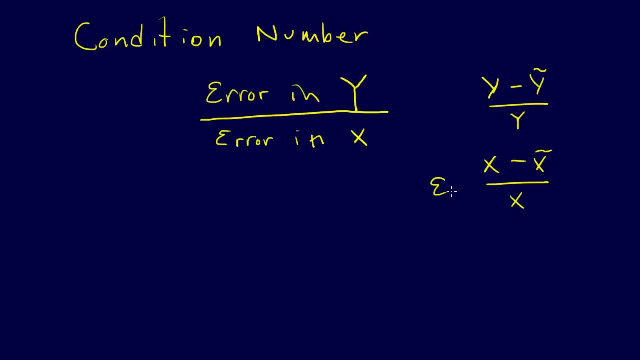 So I mean this is error in x right, This was the remember the true fractional relative error And they They derive this using first-order Taylor series expansion And what they come up with is the condition number is equal to. 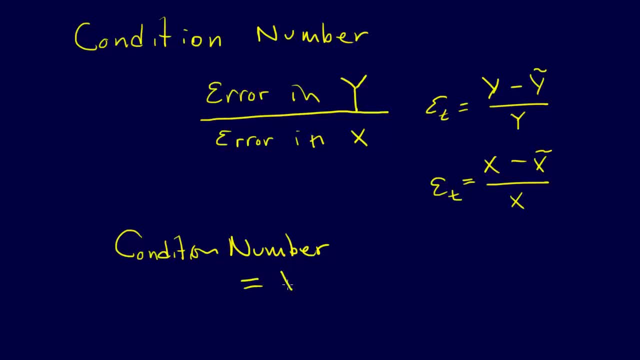 And what they say. I think they actually made an error, but Because when I went through this derivation I got something different. But they say x tilde, f of x, tilde over. I believe it's x, f of x. yeah, 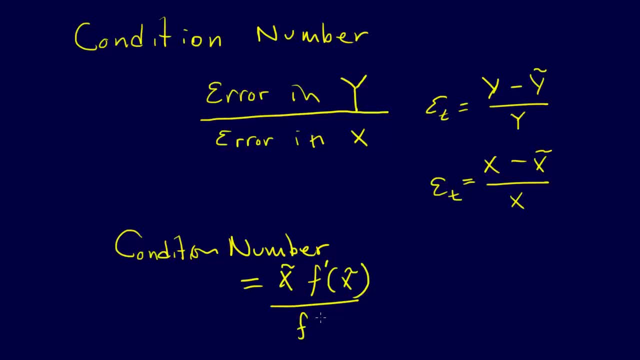 This- excuse me, this is a derivative f, And so this is how they define condition number, And using this condition number as defined here, we can- we can- get an idea for how well or ill-conditioned the problem. 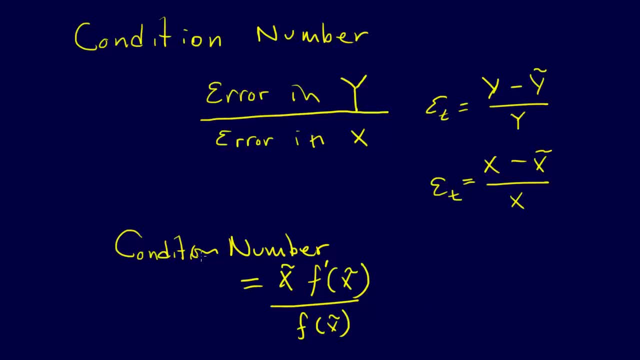 If a problem has a very large condition number, we'll just Here we go, come on. If condition number is large, then if condition number is large, then it's ill-conditioned. So we want this number to be as small as possible.